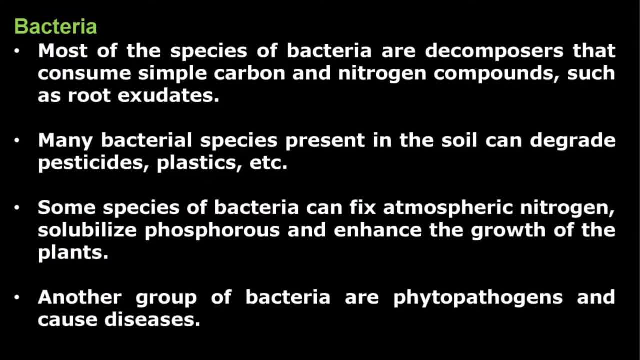 In this first, predominant microbes are bacteria. Most of the species of bacteria are decomposers that consume simple carbon and nitrogen compounds such as root exudates. Many bacterial species in the soil can degrade pesticides, plastics, etc. Some species can fix atmospheric nitrogen. 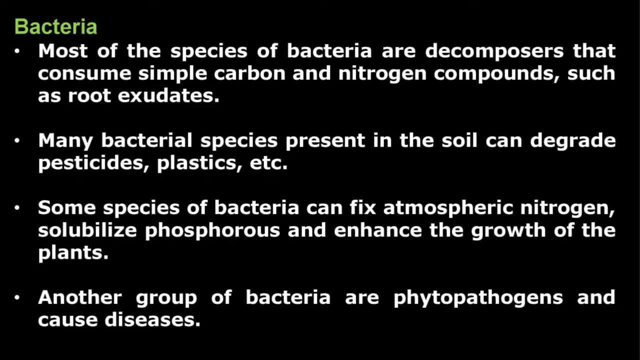 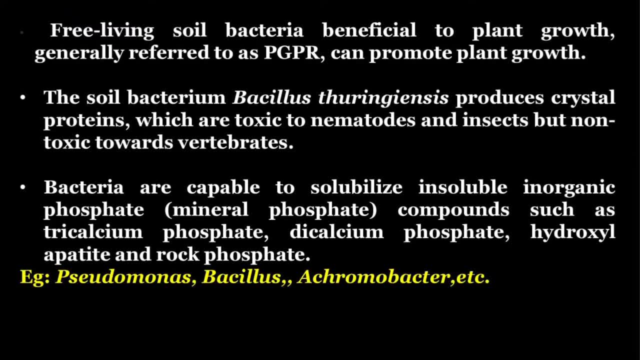 Some species can solubilize phosphorus and enhance the growth of the plants. Another group of bacteria are phytopathogens and they can cause diseases. Plant growth promoting rhizobacteria promote plant growth. The bacterium Bacillus thuringiensis produces crystal proteins which are toxic to nematodes and insects but non-toxic towards vertebrates. 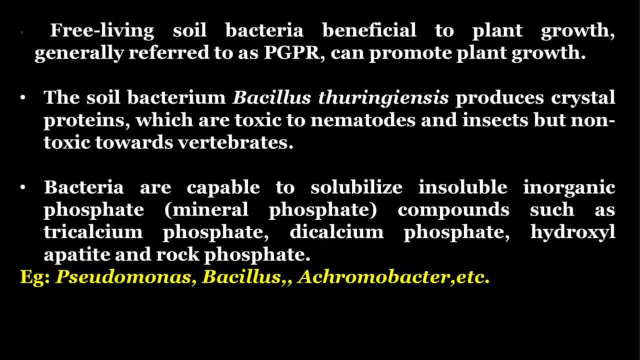 Bacteria are capable to solubilize, insolubilize and rejuvenate the soil. They are compatible in organic phosphate compounds such as tricalcium, phosphate, dicalcium, phosphate, hydroxyl apatite and rock phosphate. 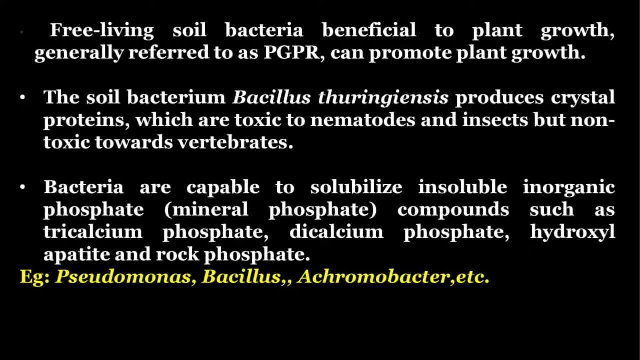 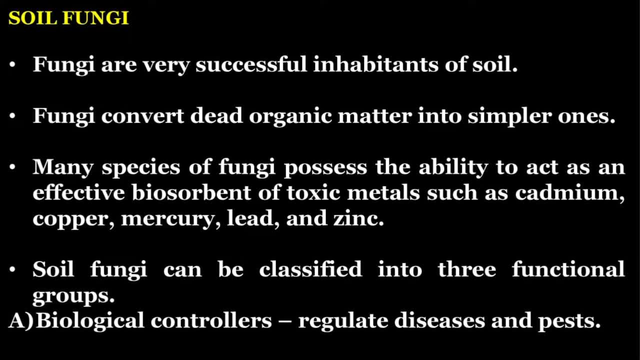 Examples for this type of bacterial species are Pseudomonas, Bacillus, acramebacter, etc. Next group of organisms are soil fungi. They are second type of microorganisms present in soil. they are very successful inhabitants of soil fungi convert dead organic matter into simpler ones. 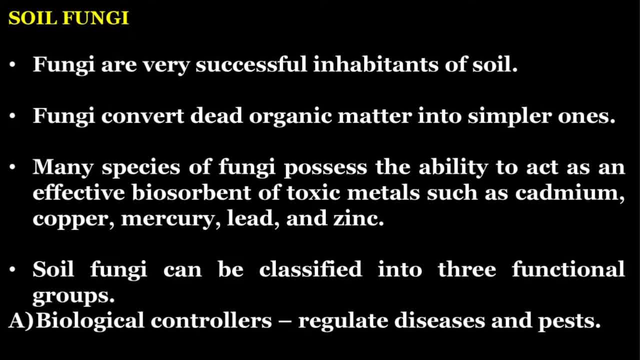 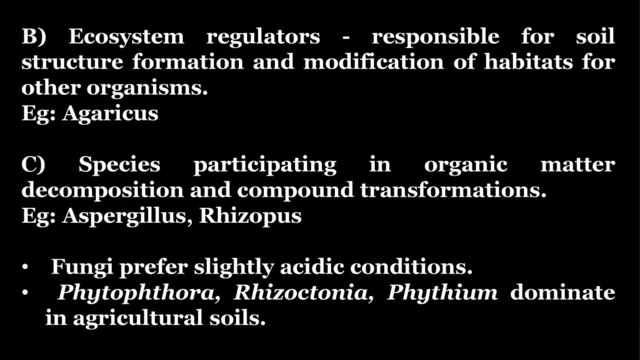 many species of fungi possess the ability to act as an effective biosorbent of toxic metals such as cadmium, copper, mercury, lead and zinc. soil fungi can be classified into three functional groups. first one is biological controllers: they regulate diseases and pests. second group of fungi are ecosystem regulators: they are responsible for soil structure formation. 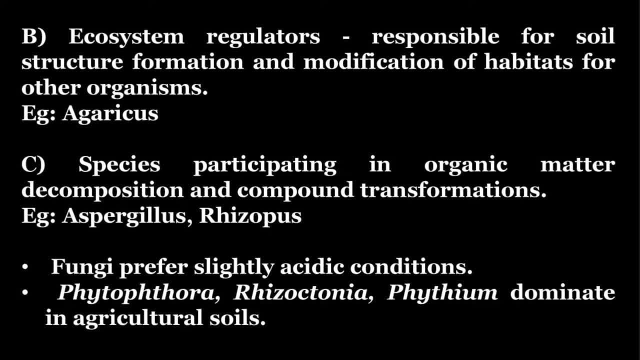 and modification of habitats for other organisms, example: agaricus. third one are species participating in organic matter decomposition and compound transformations, example: aspergillus, rhizopus, etc. fungi prefer slightly acidic conditions. phytophthora rhizoctonia pythium dominate in agricultural soils. 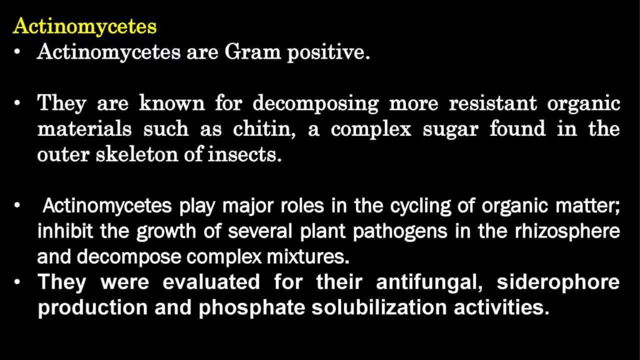 next group of organisms are actinomycetes. they are gram positive. they are known for decomposing more resistant organic materials such as chitin, a complex sugar found in the outer skeleton of insects. actinomycetes play major roles in the cycling of organic matter, inhibit the growth of several plant pathogens in the rhizosphere. 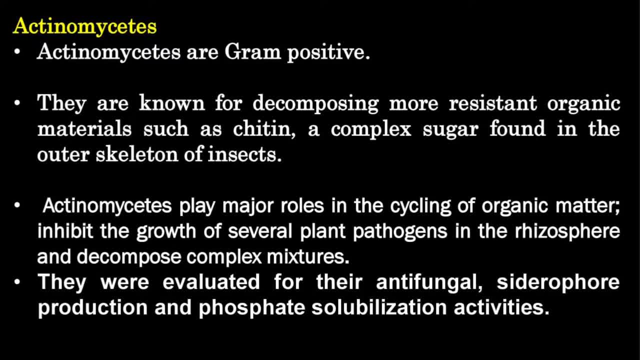 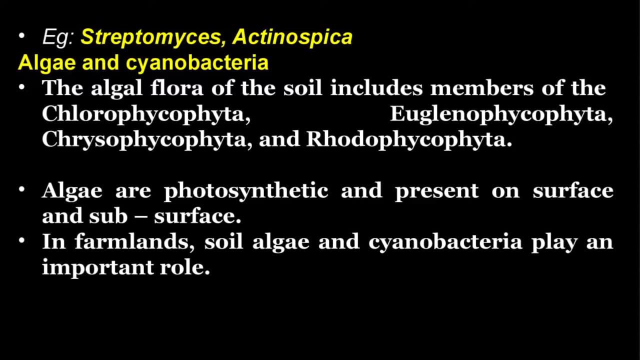 and decompose complex mixtures. they were evaluated for their antifungal activity, siderophore production and four-speed solubilization activities. example: stratomyces, actinospica, algae and cyanobacteria. the algal flora of the soil includes members of the chlorophycophyta, eugleno, phycophyta, chrysophycophyta and rhodophycophyta. 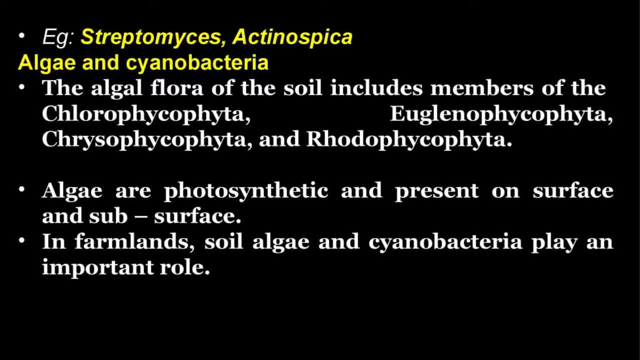 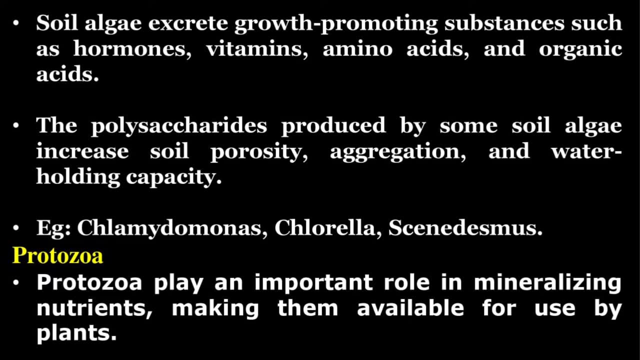 algae are photosynthetic and present on surface and subsurface. in farmlands, soil algae and cyano bacteria play an important role. soil algae excrete growth promoting substances such as hormones, vitamins, amino acids and organic acids. the polysaccharides produced by some soil algae. 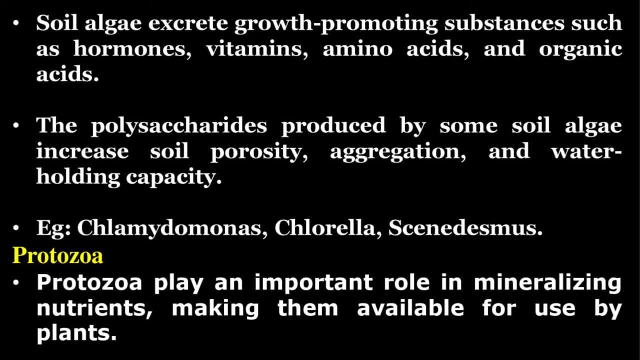 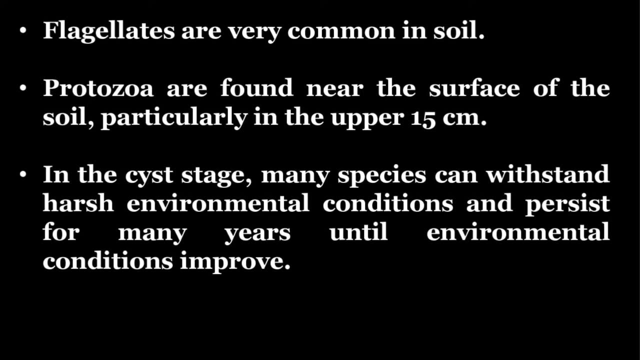 increase soil porosity, aggregation and water holding capacity. example for those type of algae are chlamydomonas chlorella senidesmus. next protozoa is an animal known by another microinheritant plant. both the plants have strong and �ed growth. all the growing tomato plants are high in ally technologies. these enjoy the Lebedo brutic Best. 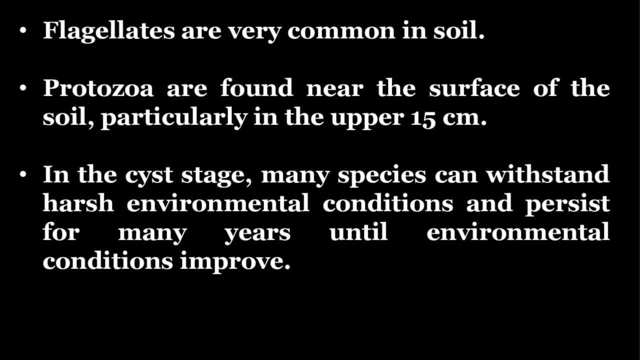 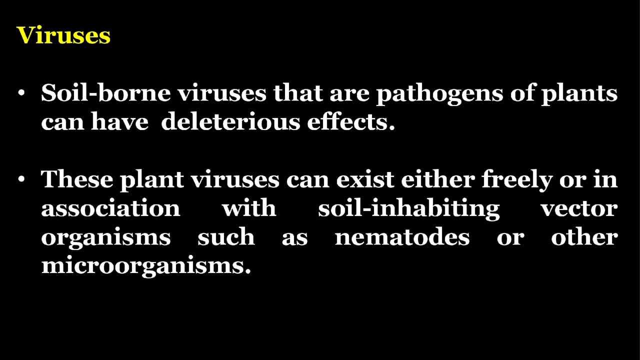 and the root-beut irgendwann, until conditions improve. Last group of microorganisms present in soil are viruses. Soil-borne viruses that are pathogens of plants can have deleterious effects. These plant viruses can exist either freely or in association with soil-inhabiting vector organisms. 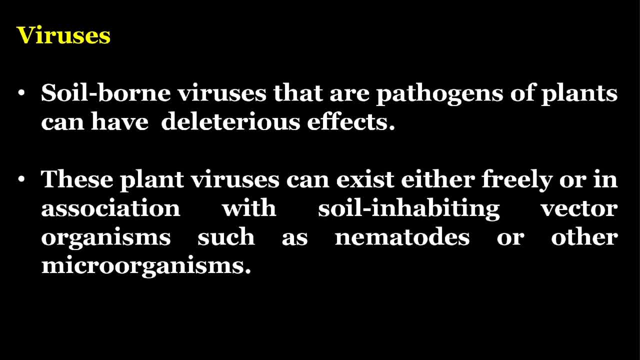 such as nematodes or other microorganisms. Subtitles by the Amaraorg community.